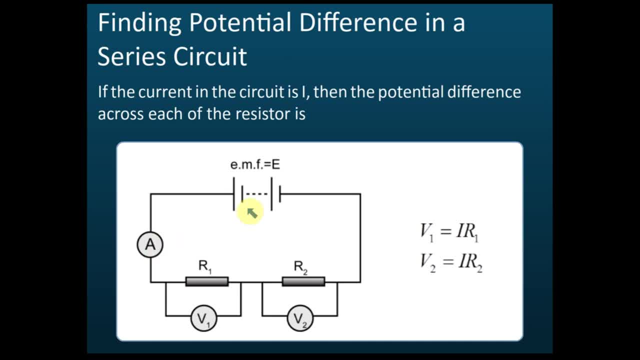 current first. okay, find the current or the readings of the emitter, the currents for in the circuit first. after you get the currents, then you can find the potential difference easily. so that is the key. yeah, that's the key. uh, to find potential difference in the series circuit you must find the current. 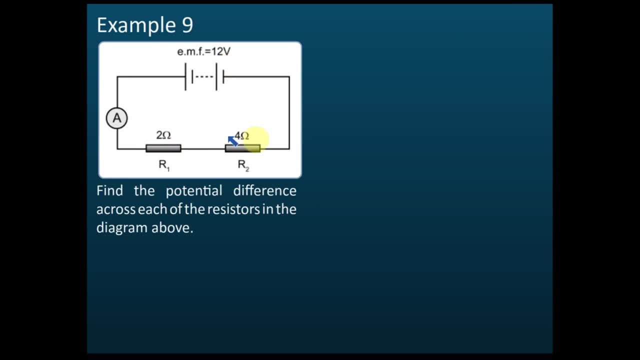 first example: nine So 12 volt, 2 ohm, 4 ohm. find the potential difference across each of the resistors. as I told you just now, you must find the Current first, and to find the currents we use the same formula, We use, or you use the same equations of V equals IR. 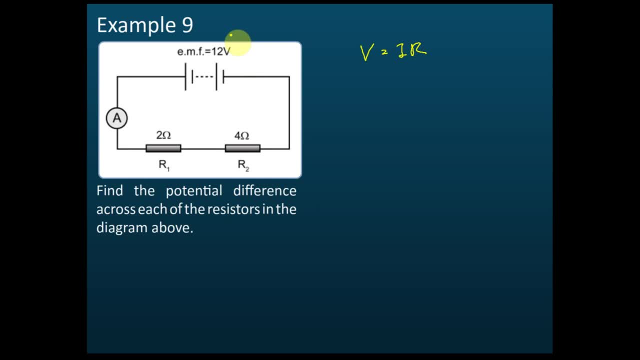 because IR. So we have this V equals to 12 volt, your 12 volt. now. now, as I told you just now, if You use this one V equal to 12 volt, you must know which two points for you to measure this V. Okay, you can choose from here to here. Okay, or you can also choose from here to here. 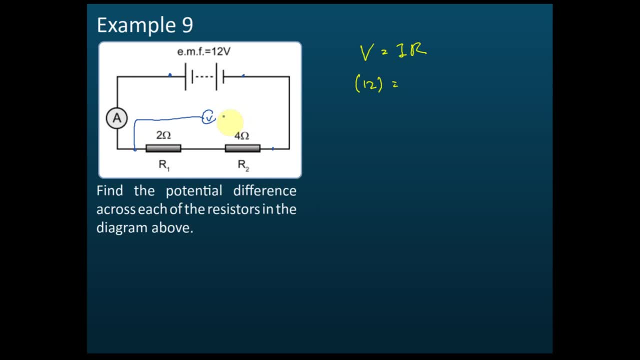 Okay, these two point and let's say we choose this one. This is for this, our V, and it's going to trial water. so if this is the V, then the resistance, the resistance will be 6 ohm, 6 ohm. so therefore the current is equals to 2. 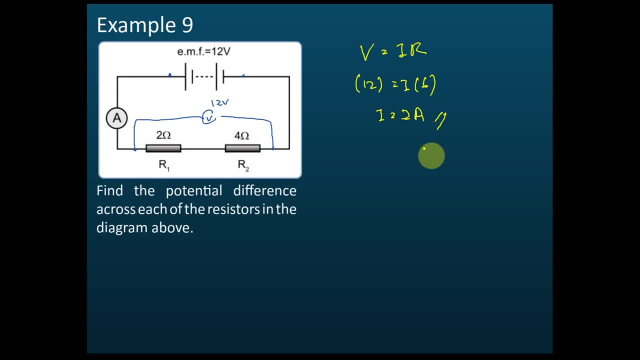 Ampere. so we get it. You must find the current first. then only you can find the Potential difference across each resistor. So now let's find the Potential difference for the first resistor, V1, V1.. So V1 equal to IR1. okay, IR1 and R1 is. 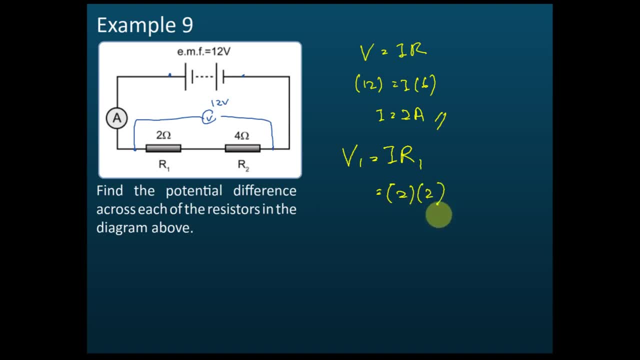 The current is equal to 2 Ampere, R1 is equals to 2 ohm. So therefore, the Potential difference is 4 volt. and how about V2?? V2, the current is still the same, 2 Ampere, Okay, but R2 is equal to 4 ohm. 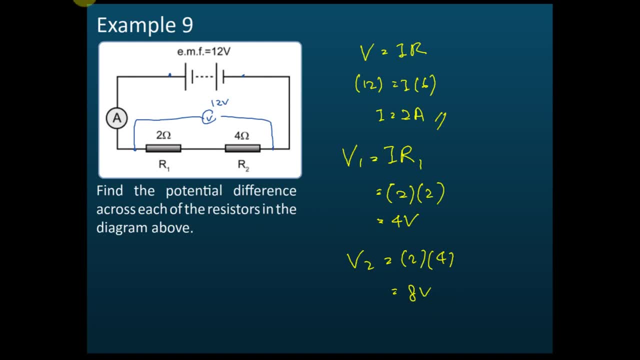 So therefore, is equal to 8 volt. so R1 is equals to 4 volt. R2 is 8 ohm. Done okay, To check whether your answer is correct or not. so you sum these two up. sum up these 2, okay, 4 plus 8, and 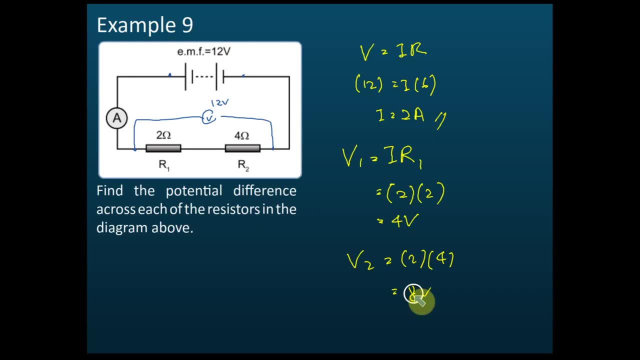 Is equal to 12 because this plus this must equal to 12. V1 plus V2 must equal to 12 ohm. done, Okay, so it's equal to 12, then that's correct. That means: So that's how we find the potential difference in a series circuit. Okay, Find the current first. That's key to solve the problem. You must find a current for this.